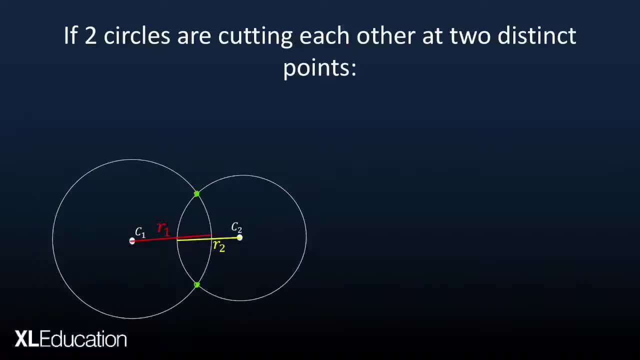 having c2. so the relationship that exists there, if two circles are touching at two distinct points, is this relationship. so the radius of one, the bigger radius minus the smaller radius, must be less than the distance between sender one and sender two and must also be less than. 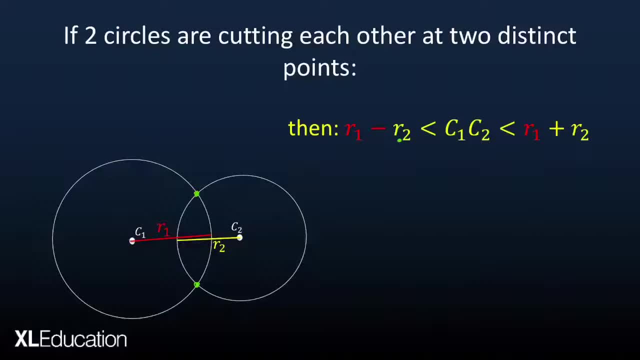 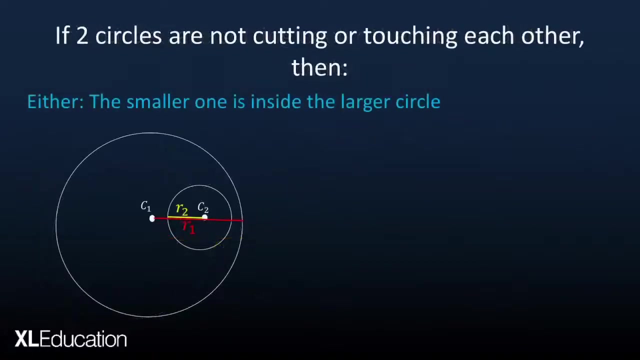 the sum of radius one plus radius two. you so the the distance between two senders must be lying between these two extremes: the difference of the two radii and the sum of the two radii. i'm going to look at a specific example where this concept is applying very soon now. the third scenario is when we've got two circles. 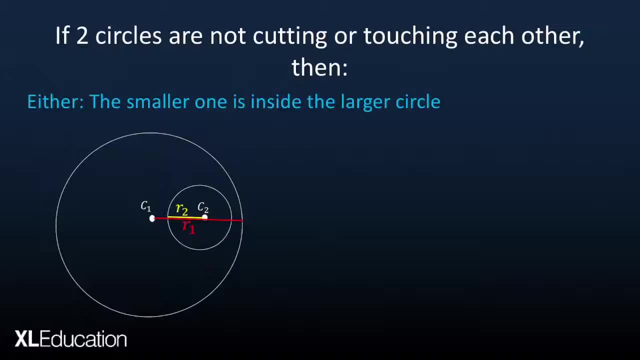 that are not cutting or touching each other. so here's the first scenario where we've got two options in R1 and R2 edge. and here we have two options: either the smaller one. the smaller circle is inside the larger circle, as shown in this diagram, and the center of the bigger circle is c1 and the 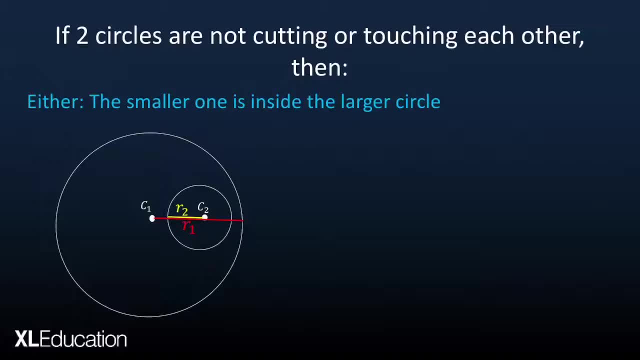 center of the smaller cycle is c2 and also the radius of the smaller circle is in yellow- is R2 and the radius of the bigger circle is R1. so in this situation we see that this distance between the two centers must be less than the difference of the Torah D. so the radius 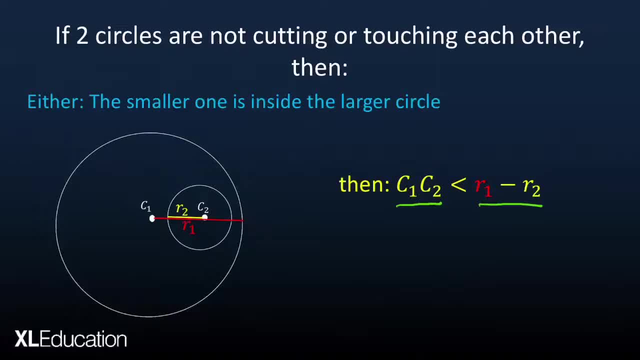 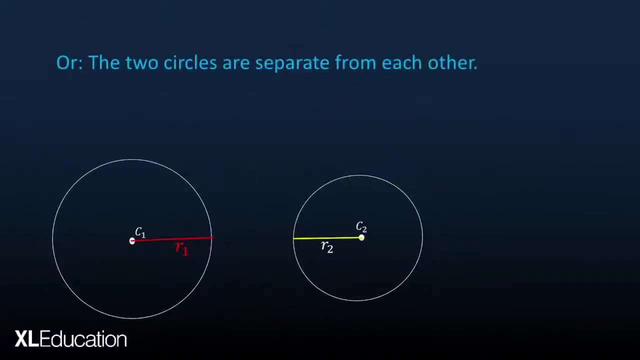 of the bigger circle and as the radius of the smaller circle must be greater than the distance from sender 1 and center 2, alright, then the next situation is: the two circles might be separated. all right, so these two circles are not, are not cutting and are also not touching each other in this particular 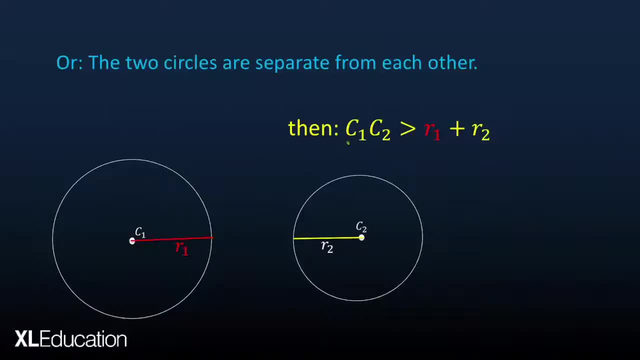 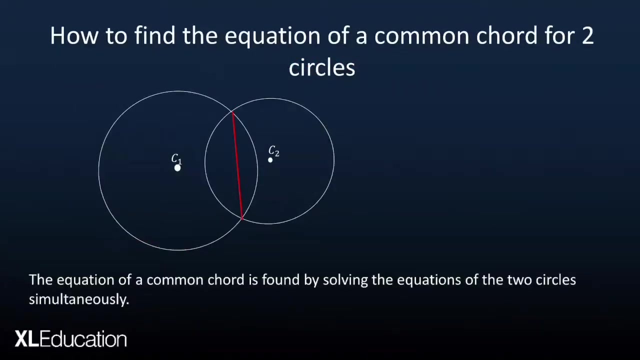 situation, we see that this- the distance between the two centers, must be greater than the sum of the Torah D. all right. now, getting to other situations, there is a situation where you are now supposed to find the equation of a common code of two circles that are cutting each other. 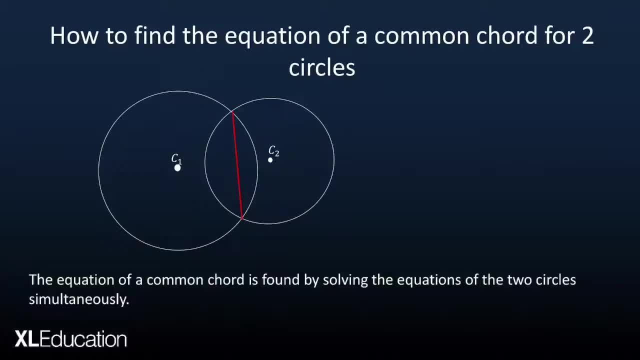 at two distinct points. so these two circles, they are cutting each other at these two distinct points. and if you join the two points, we'll see that there is a code that this two circles are are sharing. so in that situation you need to solve the equations of the two circles simultaneously. so if you do that, your 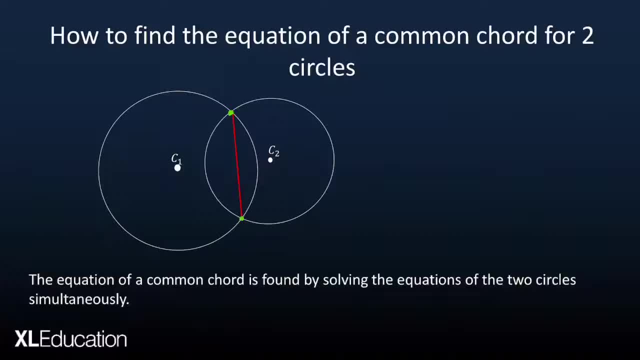 answer is going to be another equation. it will be a linear equation of the of the line that is in red. so solving the solution to this simultaneous equation is going to be equation of the form. why is equal to a something be able to reach that line? it would be another equation. if we, if we solve one equation and we share another equation, and if we do this again and then solve the solution, the answer should be ran out of the area. solution of this is much less equation. so if you solve the equation, then your answer isHaymer from y equals to a middle equation or there is no middle equation. 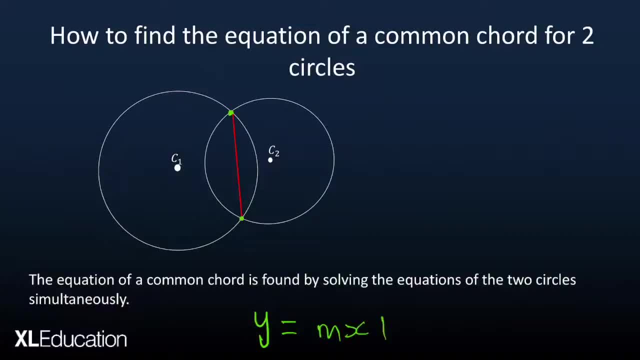 also, it has two solutions to be entered into. one solution. there will be a question about where. the answer is n. the first q equation is n스트 kanra. drawing the similar system of the two, can we see, is equal to mx plus c, because it's a straight line. i'm going to demonstrate more about this concept. 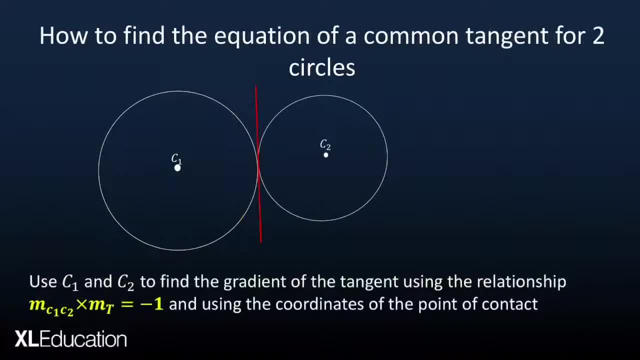 shortly. all right now. there is also a scenario where two circles are touching each other and are sharing or are having a common tangent. so a question might come and ask you: how, how do you find the equation of the line or the equation of the common tangent? so in this case, 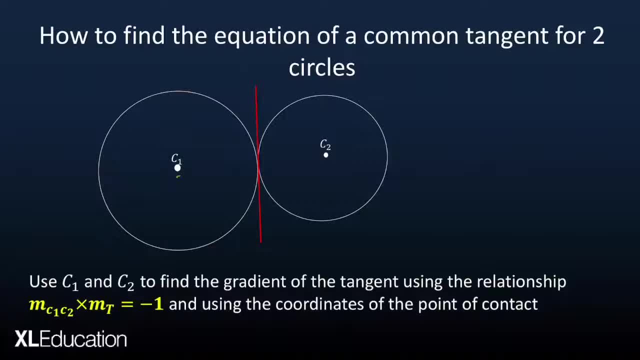 you need to take advantage of the idea that the two centers there, if you join these two centers, they will give you a line that is perpendicular to your tangent. so these two points, they can help you, you, you, to find the gradient of the, of the line joining the two centers. so the relationship that exists. 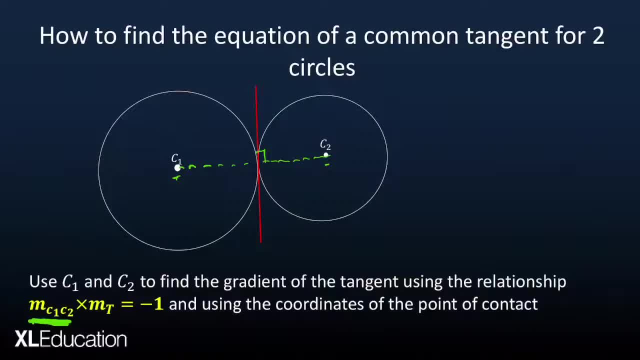 between the gradient of the, the line joining the two centers and the tangent, is that the product of these two, of these two gradients, must give you negative one. so, after getting the gradient of the of what? of your tangent, then you can use the coordinates of this point of contact of the two circles and the tangent, so that will enable you. 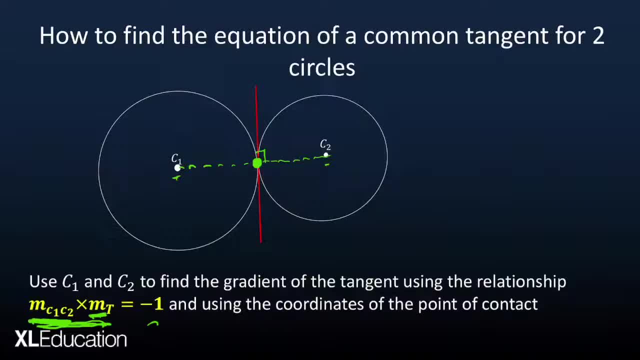 to get the equation of a tangent, and it's going to be in the form: y is equal to m x plus c. all right, so we have looked at different situations of circles interacting with each other. now we want to look at one example of a circle interacting with each other. now we want to look at one example. 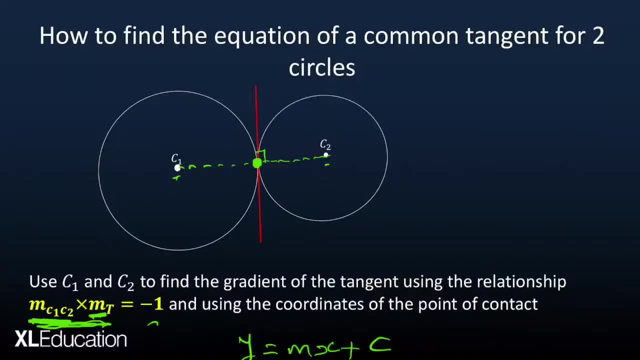 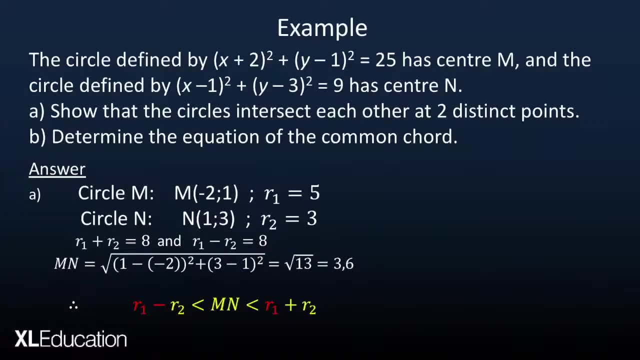 where we are applying all these concepts. so in the example we are having the circle defined by x plus 2 squared plus y minus 1 squared equal to 25 is a center m. so this is one circle with center m and the circle defined by x minus 1 squared plus y minus 3 squared being equal to 9, and this circle 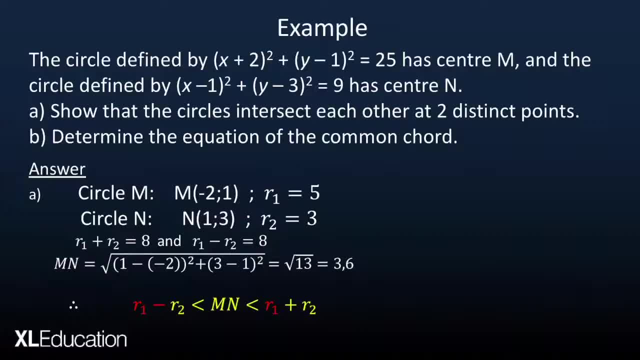 so the first question is saying: show that the circles intersect each other at two distinct points. all right, so usually when we are dealing with functions and we are talking about a point of intersection, we usually equate the two functions or we solve the functions simultaneously. but in this case, our equations, the equations of circles, they are a bit complicated, if you. 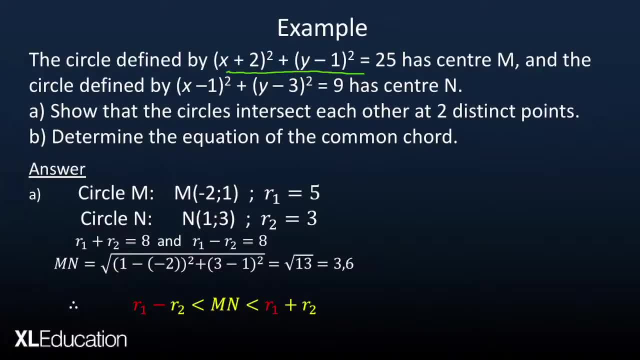 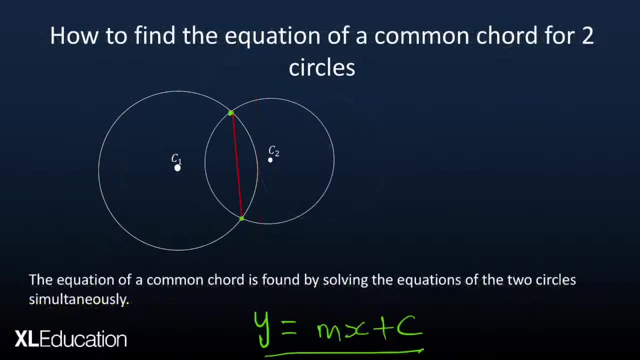 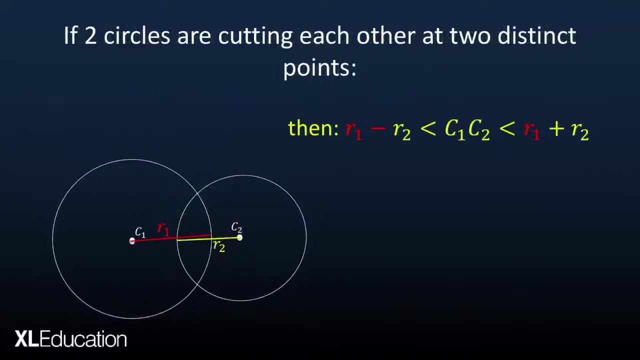 want to solve these two equations simultaneously. you see that there is a lot of work to be done there. so who can pay will just go back and see what is the condition of for two circles to touch at two distinct points, and we remember there is a condition. I'm going back to the condition. right here you are. this is the. 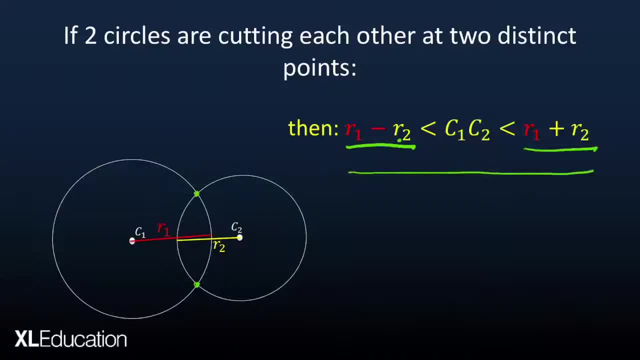 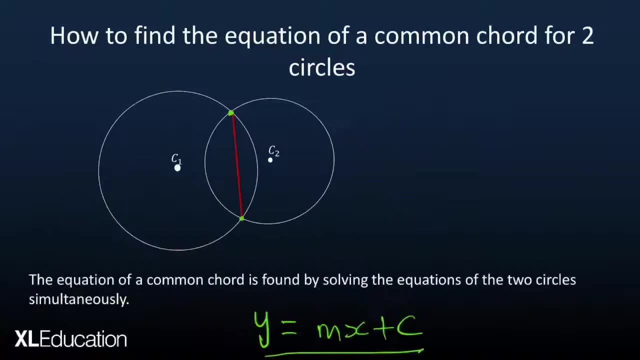 condition that we need to satisfy. if we can satisfy this condition in our question, then we can conclude that these two points, these two circles are cutting each other at two distinct points. so if you move to the question now, we will see now that the circle with sender M 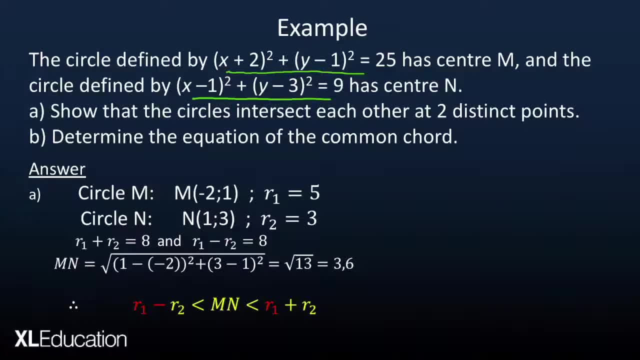 if you calculate the radius of that cycle, you see that the radius is is actually five units. and if you look at the circle with center and the radius is three units, all right. so if you say a radius one plus radius two, you see that you get an answer of eight. and if you say a radius one minus radius, 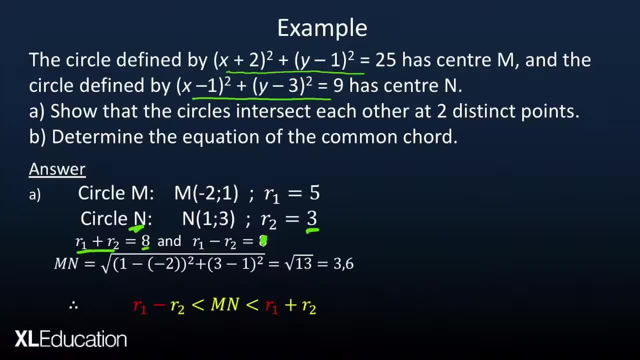 two, you get. the answer here is actually five minus three, and this gives you two. all right, so now, if you calculate the distance between the two centers, the distance M, and you discover that it gives you square root of 13, which translates to three comma six units. 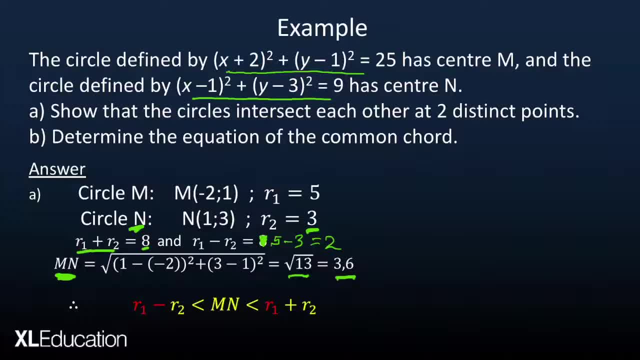 right. so now we want to compare the distance Mn to our, our two extremes, which is the difference of the two ready and the sum of the two ready. so this difference of the two ready, we remember that is actually two units, and this sum of the two ready is giving us eight units and Mn. 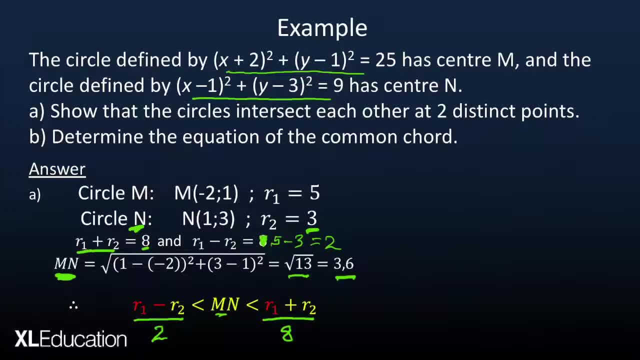 is three comma six, which is indeed between these two, these two extremes. so you can see that it is satisfying the condition that we studied earlier on. therefore, the two circles, the two circles are indeed cutting, uh, each other at two distinct, distinct points. all right, so we have answered this question. make sure you show your calculations, how you 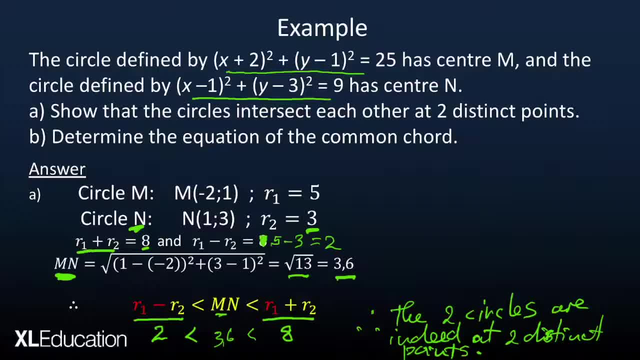 found. you find your two ready, you your sum, your difference. then you find your distance, M, and you compare that after comparing, don't keep quiet, don't just stop there. you need to go ahead and conclude, to show that this condition, this condition, here, you must show that this condition is satisfied, because that's the condition that we, we are seeking. 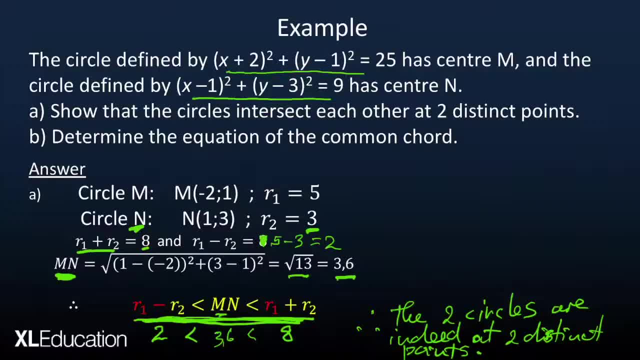 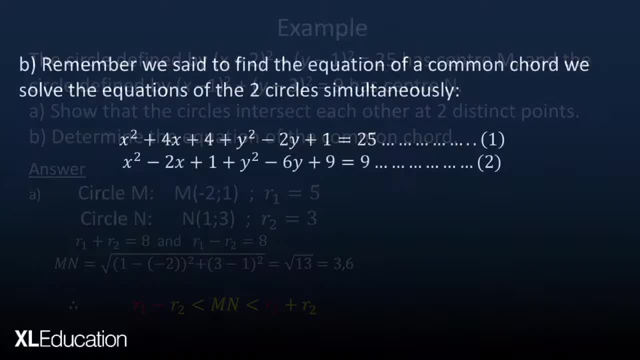 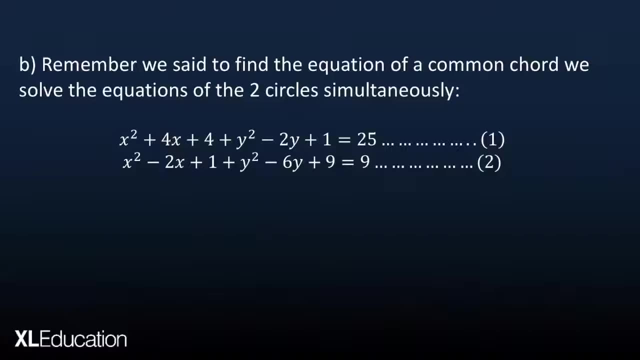 to satisfy. now let's go to question B, which is saying: determine the equation of the common code. so if you remember from our our discussion earlier, we said: to find a common code, we you have to solve the two equations of the circles. you solve them simultaneously, like I. 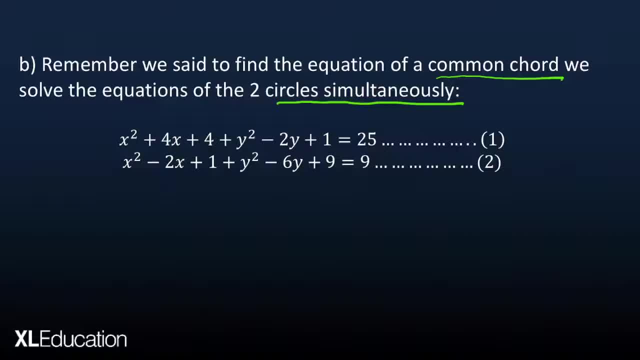 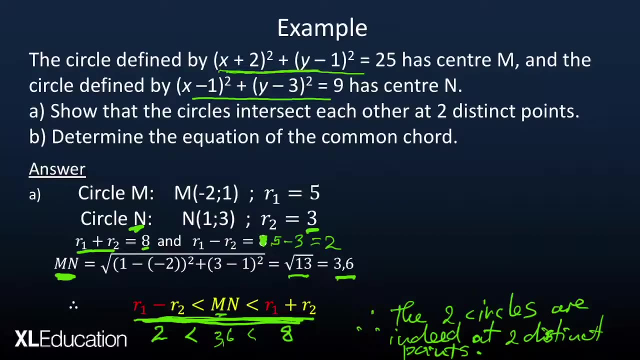 told you solving these two equations simultaneously. we need to be tactful in this case so we can use elimination method here. what I've expanded? i've expanded this equation here. if i expand it, it gives me equation number one. then this equation here. if i expand it, it gives me equation number two. so equation number one came from the first. 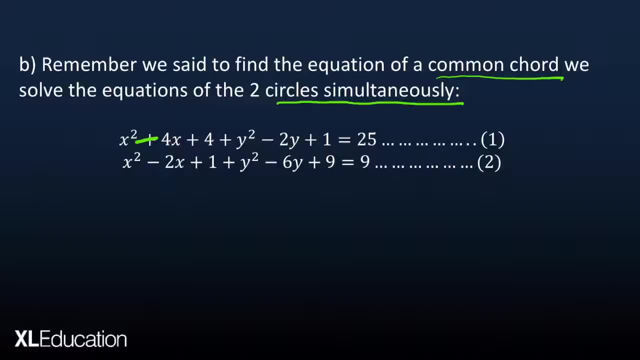 circle. equation number two came from the second circle. now i need to remove this. let me quickly remove this. uh, yeah, right. so now to solve these two equations simultaneously. by elimination. you can subtract equation one. you say equation one minus equation two. this gives you x squared and 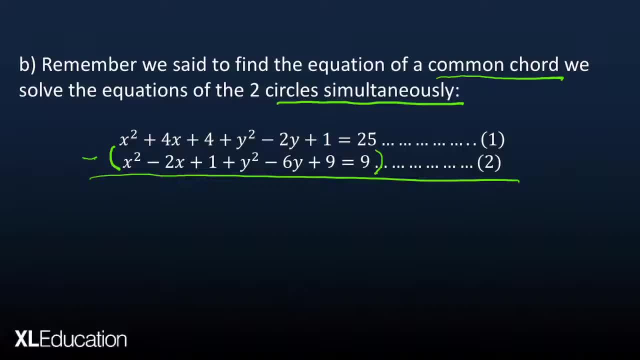 x squared, they will give us a zero there. then you 4x minus minus 2 is 6x, and 4 minus 1 gives us positive 3. then y squared minus y squared, it gives us zero. then minus 2y minus minus 6y gives us positive 4y. then we've got a 1 minus 9. this gives us negative.